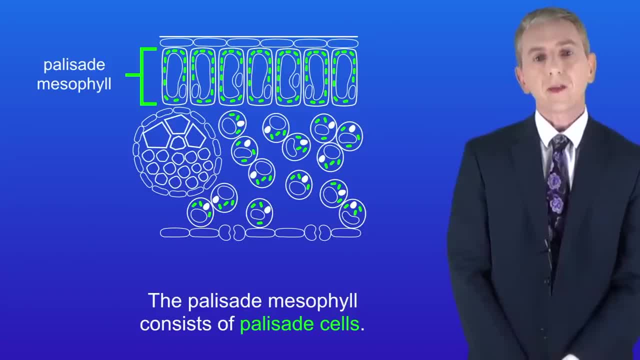 At the top of the leaf we find the palisade mesophyll. The palisade mesophyll consists of palisade cells. Palisade cells are packed full of chloroplasts. Palisade cells are packed full of chloroplasts. 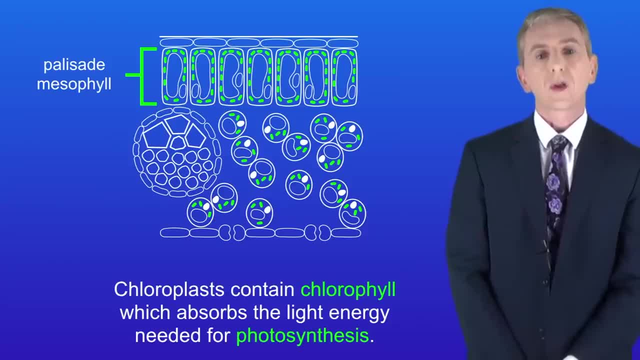 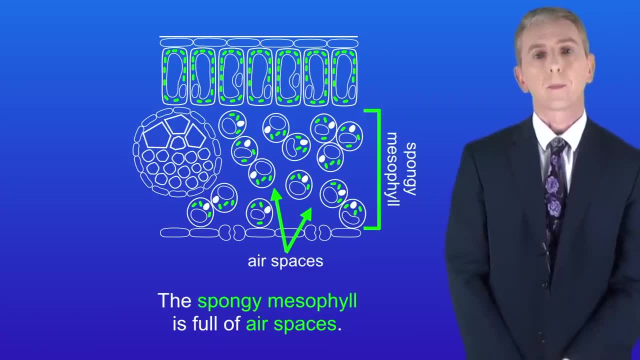 Remember that chloroplasts contain chlorophyll, which absorbs the light energy needed for photosynthesis. Now, underneath the palisade mesophyll, we find the spongy mesophyll. The key feature of the spongy mesophyll is that it's full of air spaces. The air spaces allow. 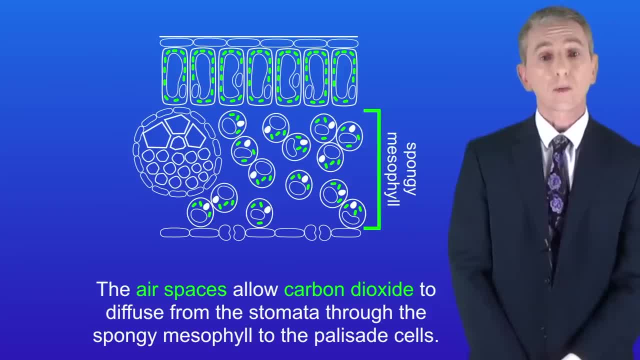 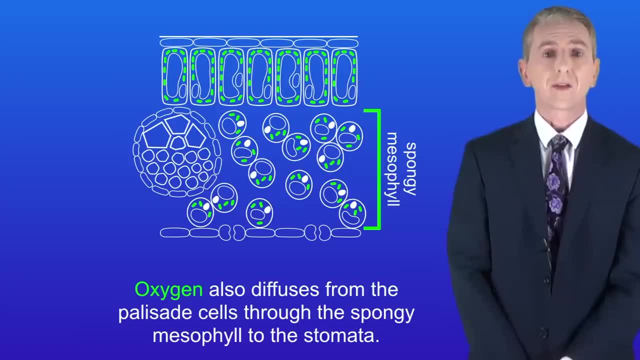 carbon dioxide to diffuse from the stomata through the spongy mesophyll to the palisade cells. like this, Oxygen also diffuses from the palisade cells through the spongy mesophyll to the stomata. There are two other tissues in the leaf that we need to look at, and these are: 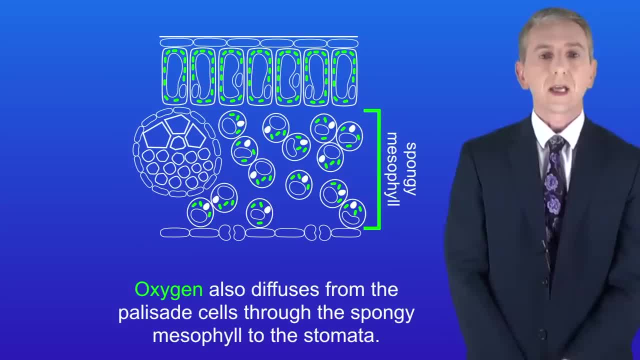 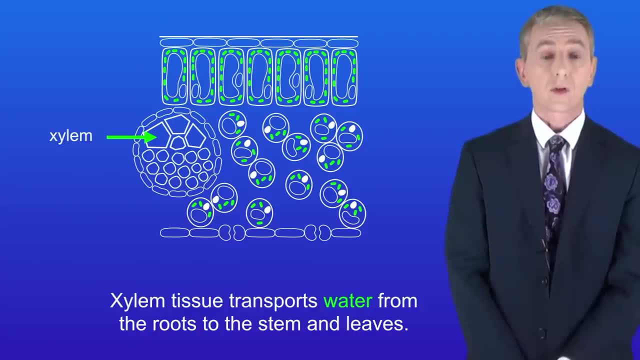 the xylem and the phloem. We've already seen the adaptations of these in the video on specialized plant cells. Xylem tissue transports water from the roots to the stem and the leaves. Some of the water is then used in photosynthesis. The xylem also transports dissolved mineral ions. 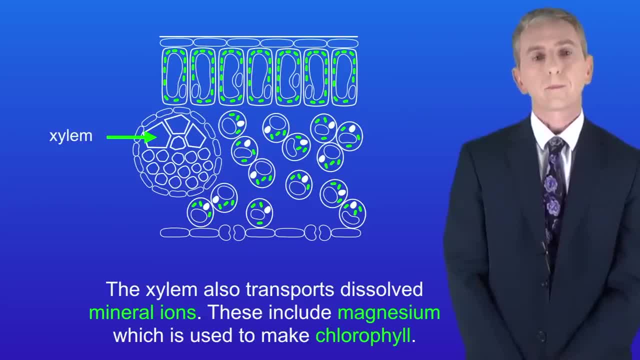 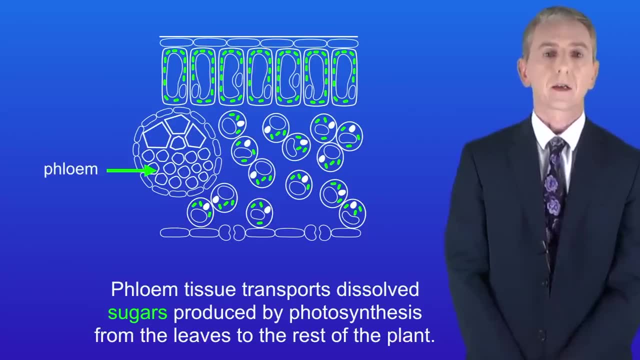 These include magnesium, which is used to make chlorophyll. Phloem tissue transports dissolved sugars produced by photosynthesis from the leaves to the rest of the plant. The sugars can be used immediately. for example, glucose is used in respiration. The sugars can also be stored. 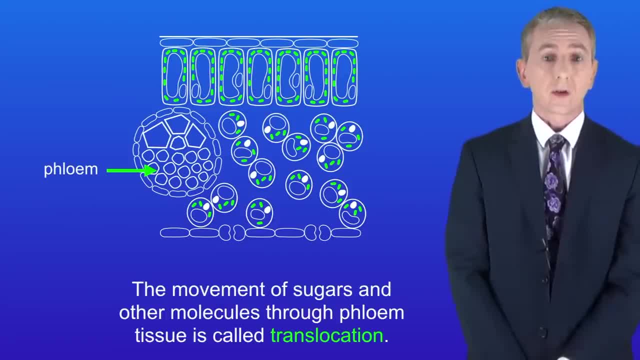 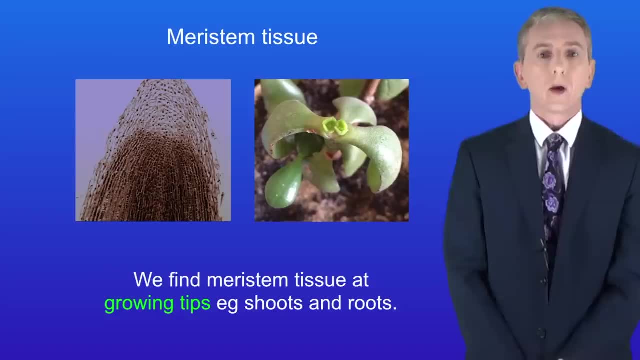 for example, as starch. Now, the movement of sugars and other molecules through phloem tissue is called translocation, and it's important that you learn that. Okay, the final type of plant tissue we need to look at is called meristem tissue. We find meristem tissue at growing tips, for example, shoots. 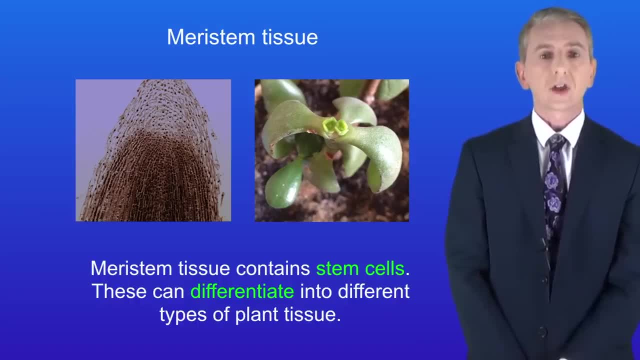 meristem tissue contains stem cells. These can differentiate into different types of plant tissue and, again, we looked at stem cells in a previous video. Remember, you'll find plenty of questions on plant tissues in my vision workbook and you can get that by clicking on the link above. 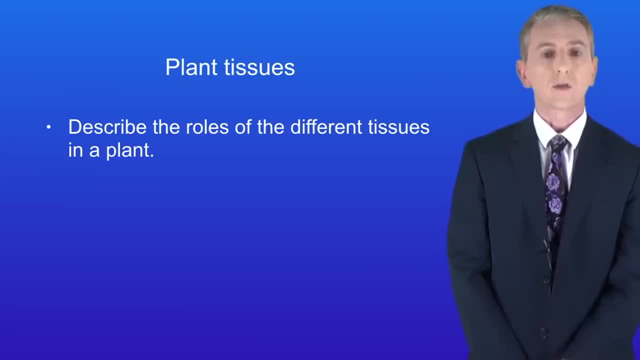 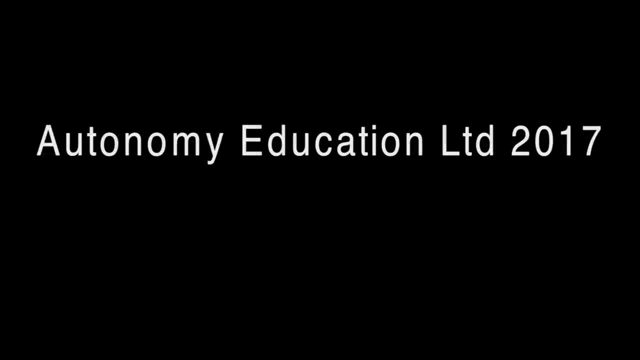 Okay, so hopefully now you should be able to describe the roles of the different tissues in a plant. Thank you so much for watching. I hope you enjoyed this video and I'll see you in the next one.